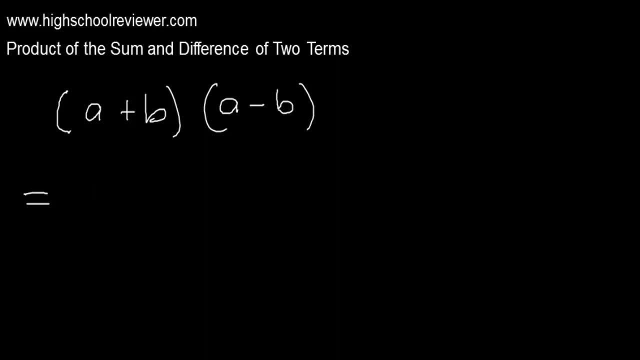 So the first step is just to square. We will just square the first term And we have here A squared, And then we will subtract, So the square of the first term minus the square of the second term, And this is our answer. 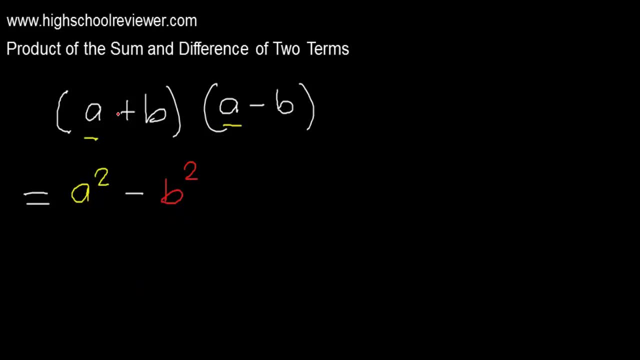 It is this easy Again, remember: the product of the sum and difference of two terms is equal to the square of the first term minus the square of the second term. For another example, we will try to have here a reverse. So A minus B will be the first quantity and A plus B our second quantity. 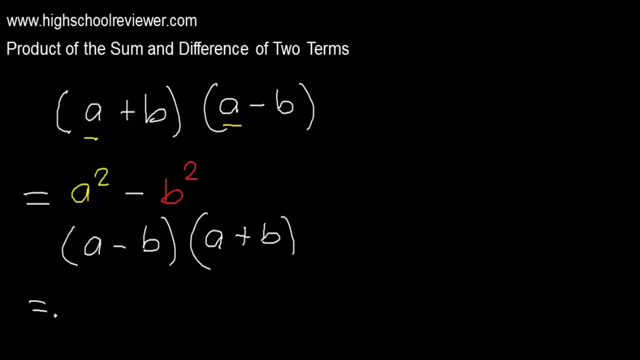 No matter if we interchange the two quantities, if minus sign will come first as the plus sign, the answer would still be the same: It would still be the square of the first term minus the square of the second term, So it would still be A squared. 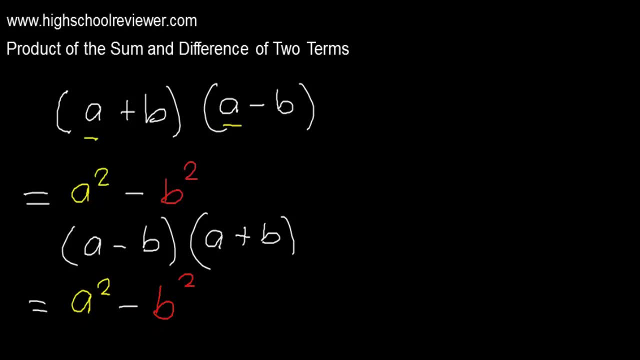 It would still be A squared minus B squared. This is our answer for the quantity of A minus B multiplied by the quantity of A plus B. Let's have another example. Let's say we have the quantity of K plus 5 multiplied by the quantity of K minus 5.. 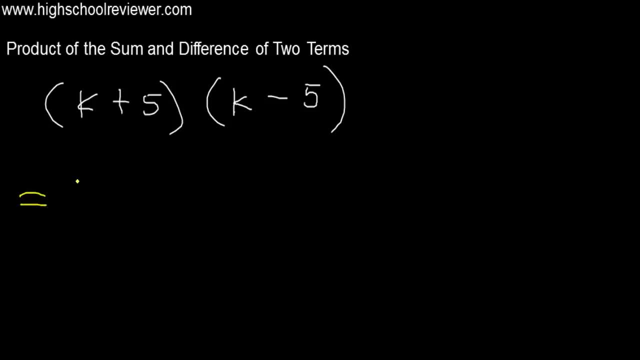 It would still be the square of the first term. Our first term is K, So that will be K squared minus the square of our second term. Our second term here is 5.. So K squared minus 5 squared, This will be K squared minus 5, raised to 2.. 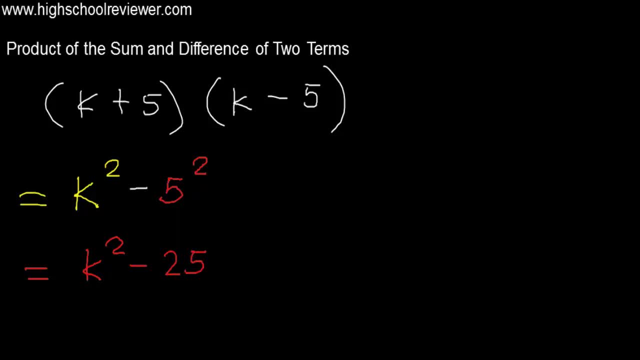 That is equal to 25.. So K squared minus 25 is our answer. Let's have another example: Our P of positive 5A minus 6B And multiply this by the quantity of 5A plus 6B. What will be our answer? 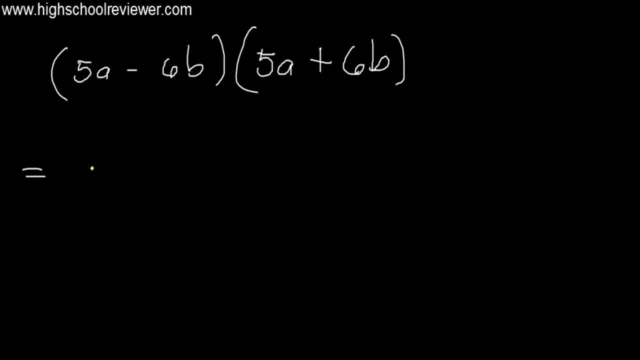 The steps would still be the same. It is still the first term, or the square of the second term, Or the square of the first term. This will be 5A raised to the power of 2, minus the square of the second term. 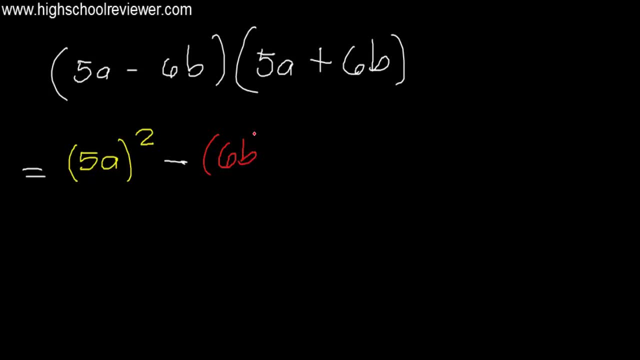 Our second term is 6B and raised to the power of 2.. And let us expand this. We will have here 5 raised to the power of 2.. That is 25A squared Minus 6 raised to the power of 2.. 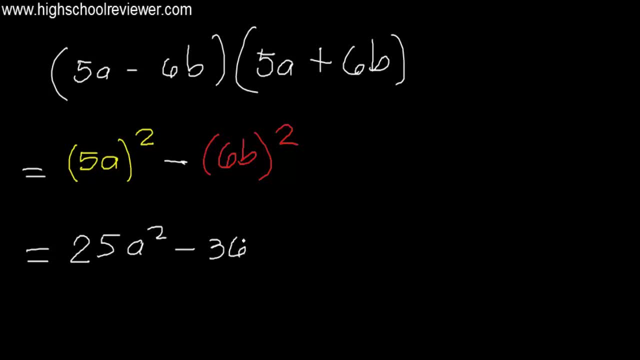 Minus 6 raised to the power of 2.. That is 36B raised to the power of 2B squared. And this is our answer. And then let's have another example. We will have here the quantity. We will have here the quantity of. 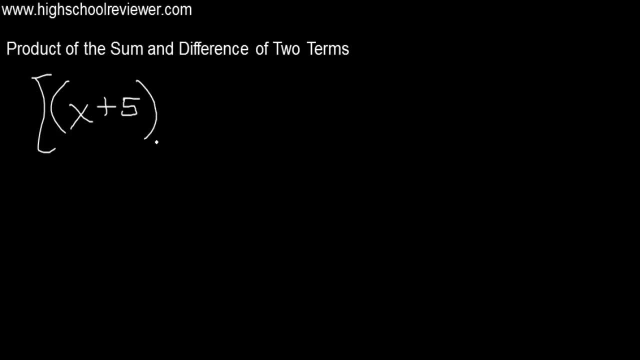 The quantity of X plus 5.. Minus 10.. Multiplied by the quantity of another quantity: X plus 5 plus 10.. As you can see, here our first term is a quantity, So our first term is X plus 5.. 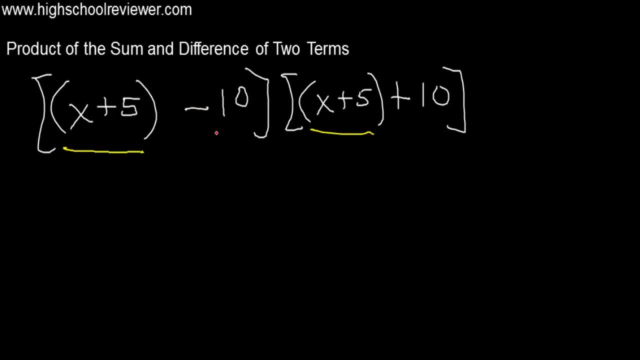 And our second term is 10.. Okay, So the same rule applies Again. our answer would be the square of the first term- So this will be our first term- is considered as X plus 5. And it is raised to the power of 2 minus the square of the second term.